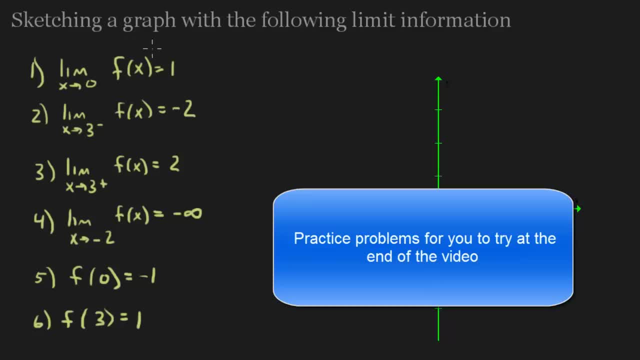 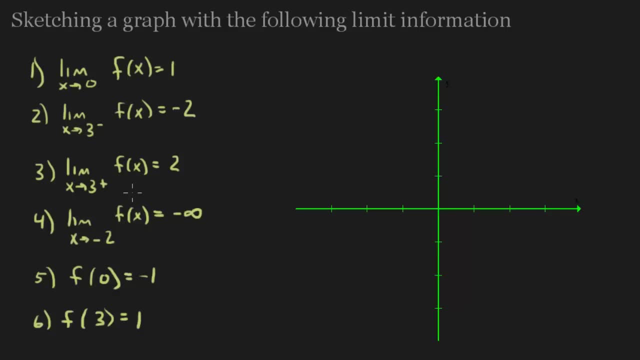 Hello, in this video we're going to sketch a graph given the following information about the limits. Now notice: the first four pieces of information have to do with limits and the last two are actually y values. So these are function values. That means they are actual closed dots on my graph. 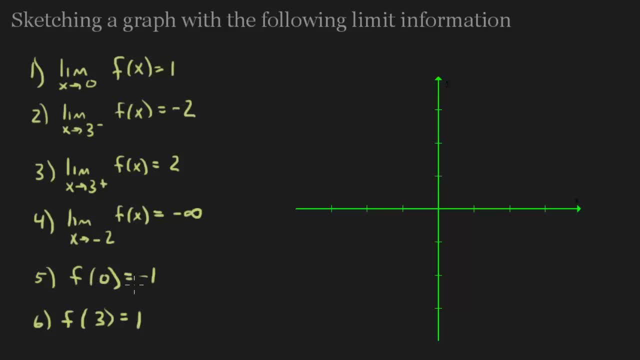 So let's start with those Now. f of 0 equals negative 1.. That means I'm graphing the point or I'm plotting the point. 0, negative 1. Because that's my x value right here and this is the y value. 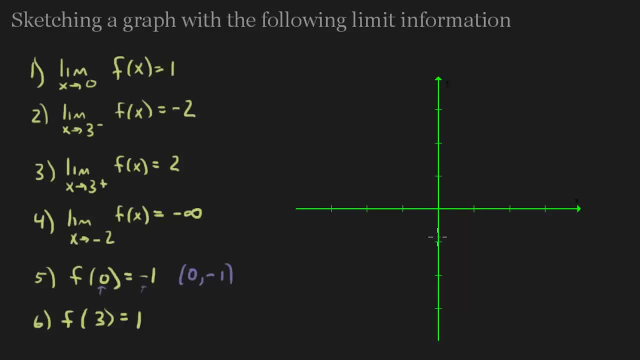 So 0, negative 1.. So let's go ahead and plot that now. Alright, next one is f of 3 equals 1.. So that makes the point 3, comma 1.. So let's go ahead and plot that. 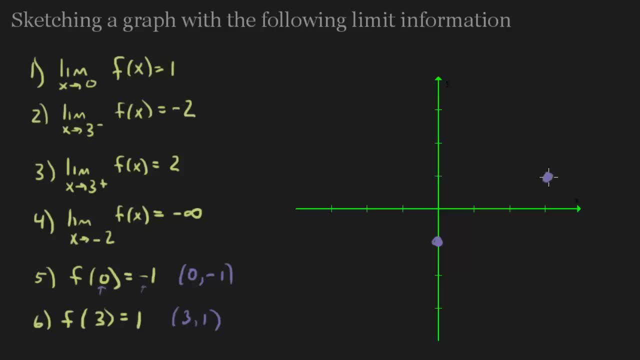 That puts me right there. Now, because those are actual, real function values, they're given closed dots. Let's go ahead and do number 1.. Now, if you remember from previous videos, limits are like hypothetical y values. They're what I expect the y value to be. It may not actually be the point there. 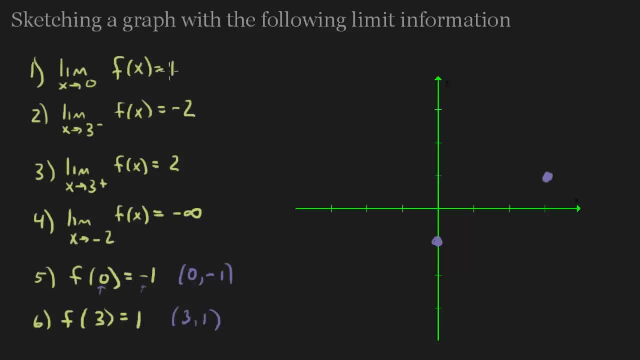 but I expected it to be that point. So when you look at this, you can actually think of it as the point where the x value is approaching 0 and the y value is approaching 1.. So I can go ahead and try plotting the point 0, 1.. 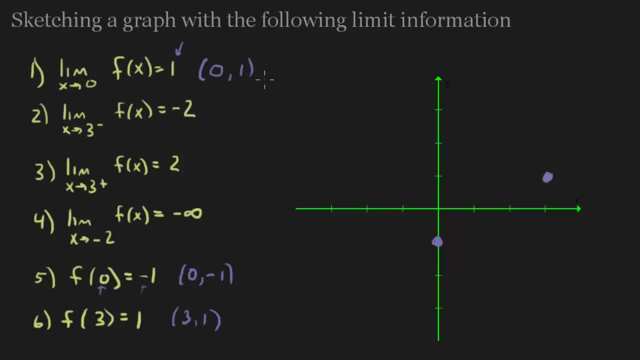 But the problem is that a limit is not a real point, So what we would do is we would put an open dot there at 0, 1.. Now, because limits were talking about what was happening when I was getting close to 0, right. 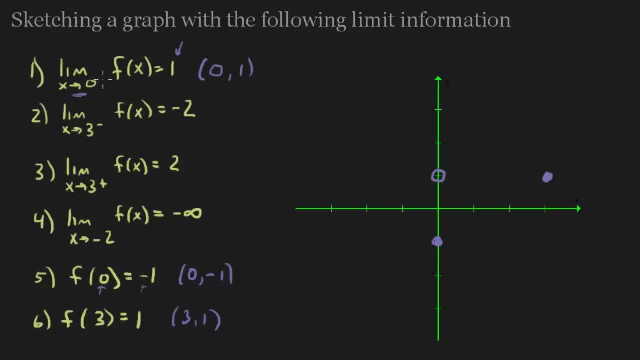 Getting close to 0.. I looked at the direction and I don't see a direction. That means this is a general limit and it means if I were to come in from the left and right, so coming in from the left and coming in from the right, I would have expected this point. 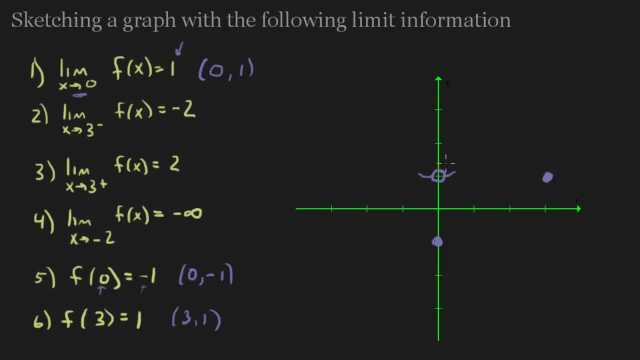 Alright. so now I've actually graphed what my function should look like. with this information right here, Let's go ahead and try the exact same thing here. The limit of the function as x approaches 3 from the left is negative 2.. 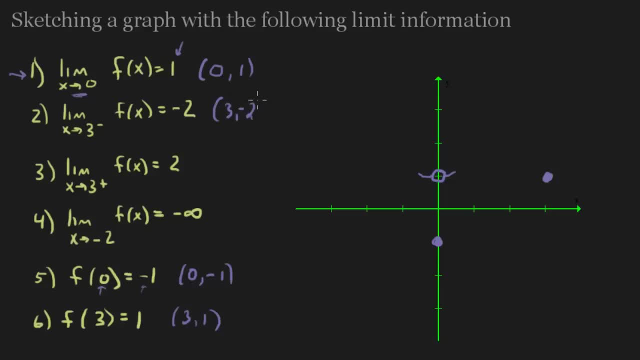 So I'm looking at the point 3, negative 2.. So if I were to approach 3, where's 3? Right there. If I was approaching 3 from the left, I would have expected this point 3, negative 2.. 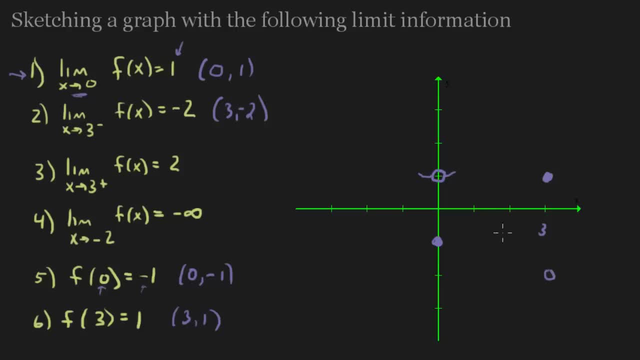 Now I'm not actually going to try connecting dots because I'm not actually sure what happens here yet, Because I still have other information. So what I'm going to do is I'm just going to plot the point and I'm just going to draw a little tiny line out from this way. 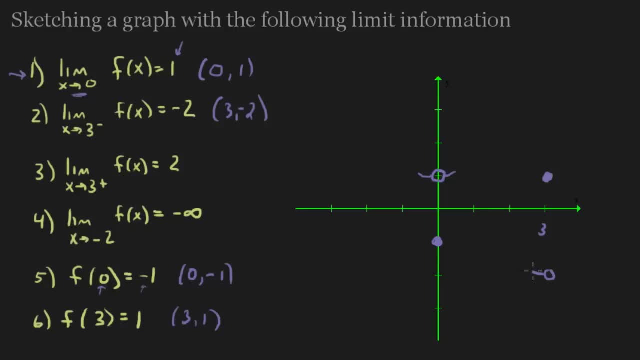 So that reminds me that when I'm coming in approaching 3 from the left, I should get- or I should look like this: Alright, next one- 3 from the right. I'm approaching 2, so that means I'm having. 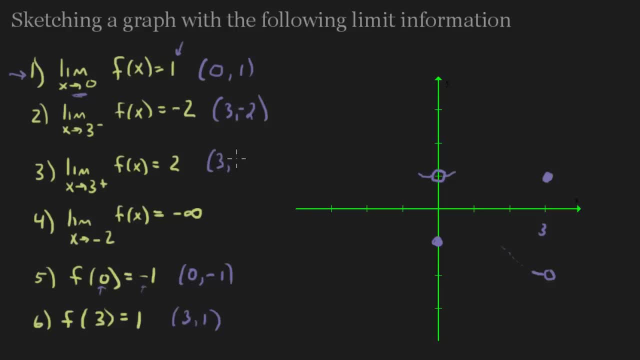 and, if you haven't figured this out yet, all limits end up being closed dots. So we have 3, 2.. So let's go ahead and plot 3, 2 as an open dot, Because the direction is a right-hand limit. 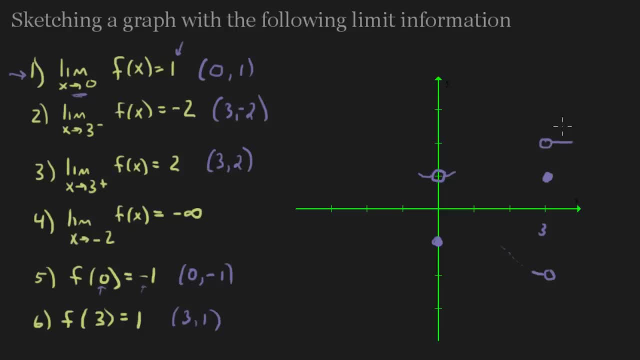 I'm coming in from the right. So far, this is what I have. Now, onto the last one, I have the limit of my function as x approaches negative 2.. So here's negative 2. And it's going to negative infinity. 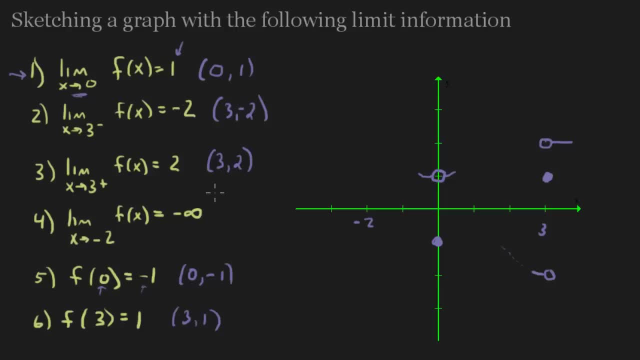 So remember that negative infinity isn't an actual y-value, so there's not anything we can plot. But when the limit approaches infinity, it means that it has that vertical asymptote. So let's go ahead and plot a vertical line, And I want you to think of limits as when they approach infinity. 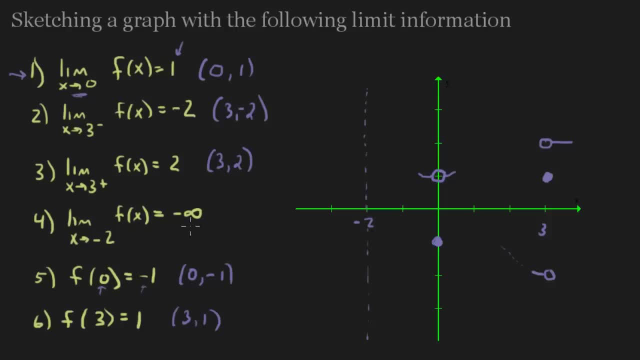 as kind of like the behavior of the function. It means it's not approaching a y-value, but it's approaching an asymptote, a vertical asymptote, And because there's no directional limits on this, it means it's approaching negative infinity from both the left. 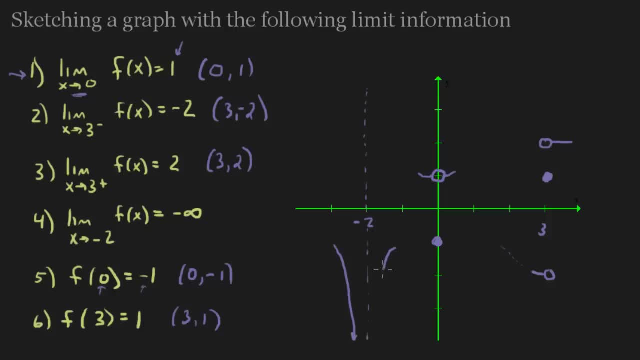 so going like that, and the right. so coming in from the right, I'm also going to negative infinity. So now I have all the following, or I've actually dealt with all of these pieces of information, So I have something that looks like this: 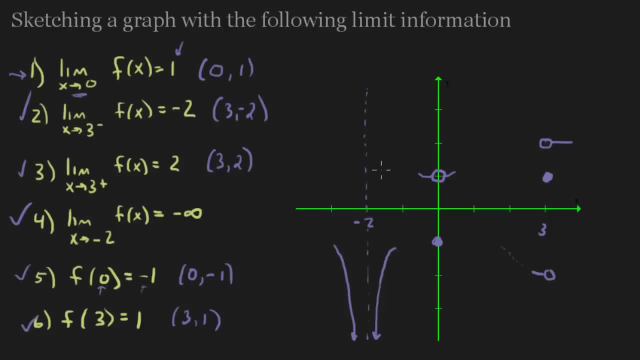 So what I'm going to do is I'm just going to connect the dots. So let's take a look We have. I mean, I could do something like this. Now this has to connect to. now what happens is people get confused. 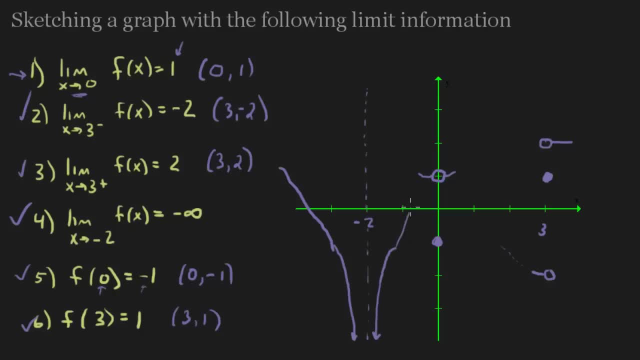 Am I connecting here Right Or am I connecting up here And remember that this is a limit? This was just a y-value. Now limits are telling me where I'm coming from, So I'm approaching this point from the left, so I would actually connect. 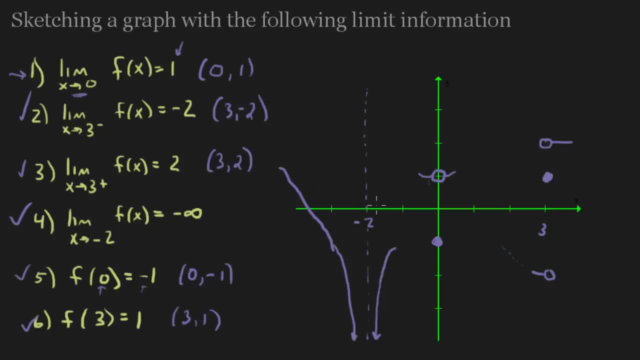 Let me do it with a different color here. So I'd do something like this, And then I would approach this point from the right, and so I'm coming in here. So where would I go? I can go here, here or here. 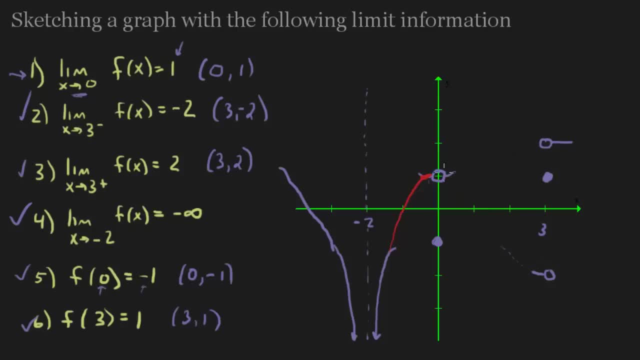 It depends on what the limit was doing. Alright, I was approaching 3 from the left. I was approaching this point, so I would go ahead and come down here and connect There And finally I have this and I'm just going to go out here. 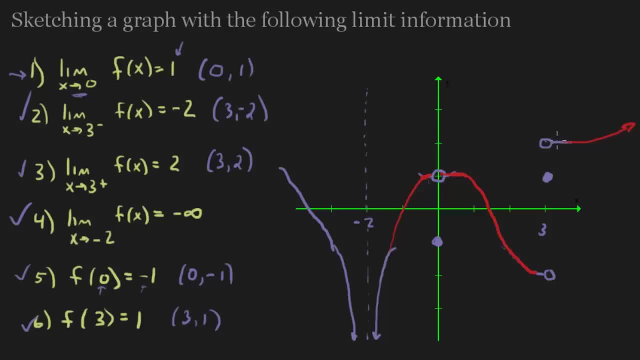 That's why I plotted like these open dots with like tiny little lines to remind myself that's how I'm actually going to connect my points. These closed dots tell me nothing about what's happening from like the left and right. So when you plot those, that's all you're getting. 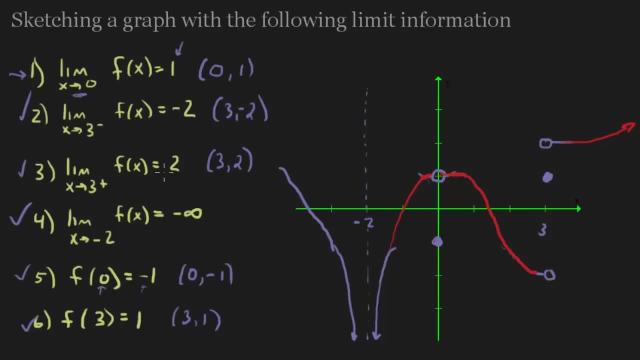 The limit is really going to tell you how your graph is going to look. Now I just I want to make this graph a little prettier, so I graphed it, and this is what it looks like when it looks all nice. Now what you should do is, after you graph, something like this: 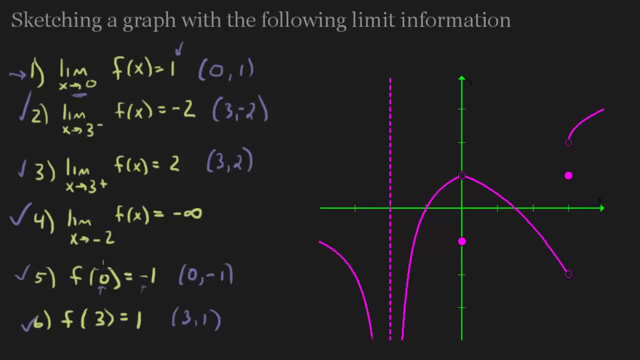 to go back through your conditions and make sure that they all match. So, for example, f of 3 equals 1.. Alright, 1, 2, 3, 1.. There it is. Does the limit as x approaches 3 from the left?